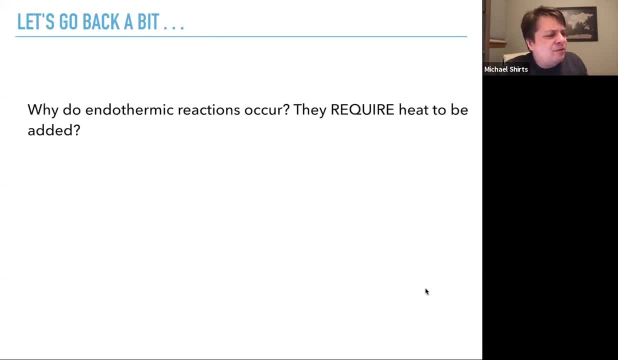 up in energy, so it needs an energy input. So why do endothermic reactions occur? I mean they require heat from the surroundings to move in. for that reaction to be possible to happen, They require heat to be added. It seems like that. that would not. you could. 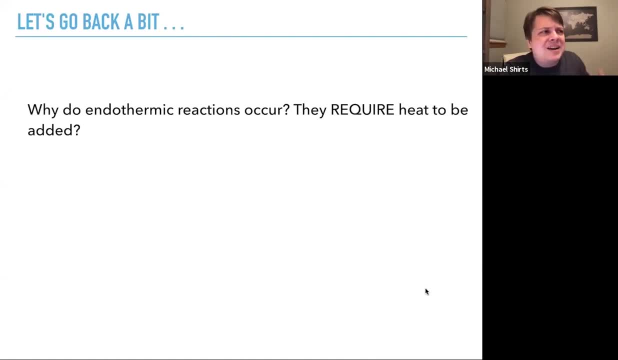 imagine that if it heats something up, then it would happen. but why would there be endothermic reactions that happen just on their own? And so one phrase, a term used here is spontaneity, the idea of spontaneity, the idea that once a reaction starts, it proceeds without continuous. 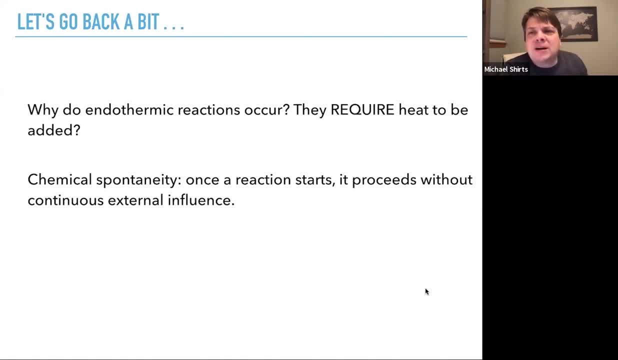 external influence, like heating it up. So really, when we talk about a reaction occurring, we talk about it being spontaneous or not. So an endothermic reaction that I posted a video of before. we usually do a demo of it, but, alas, Barium hydroxide octahydrate plus ammonium nitrate reacting to produce barium. 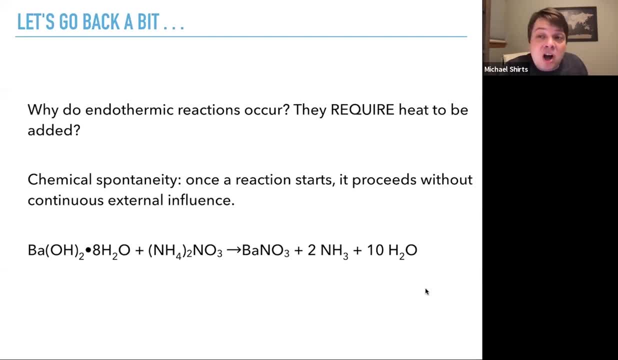 nitrate plus ammonia plus H2O And, if you recall, this was an endothermic reaction. It actually sucked up enough heat from the environment that it actually could freeze the beaker to a wooden block. So it's an endothermic reaction. The change in enthalpy is positive. standard change of enthalpy. 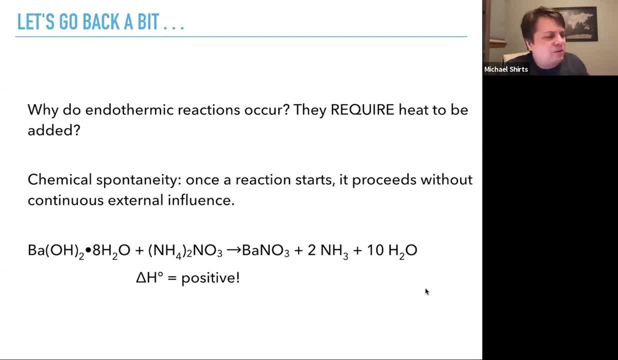 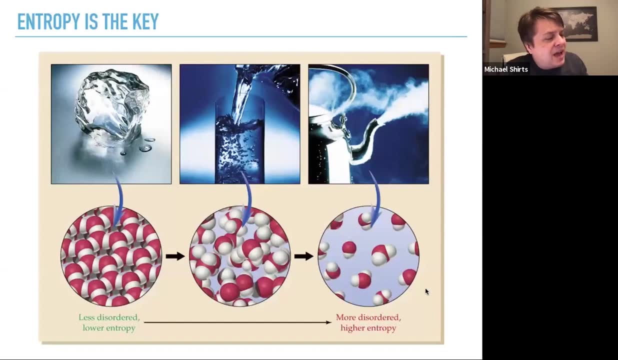 is positive. And so what is it that makes this reaction happen? How does it be? Why is it spontaneous if it's actually climbing in energy instead of dropping down in energy? And the key to this is entropy. So we'll be talking a lot in the next two lectures about entropy, and especially 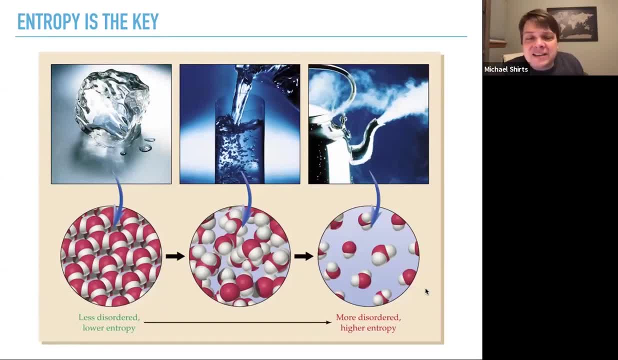 how to quantify it. So let's, we'll start on that this lecture. We won't really, we won't really sort of complete the story. We'll never quite complete the story. We won't get a full picture of the story until the next lecture. So entropy is essentially a measure of disorder. It's a little. 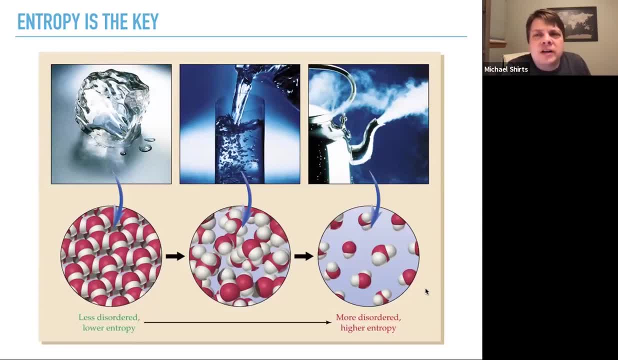 more complicated than that, but entropy as disorder is a good way to think about it. a lot of times, For example, ice does not have very much entropy because the water molecules are locked into this hexagonal arrangement where they're making as many hydrogen bonds as possible. 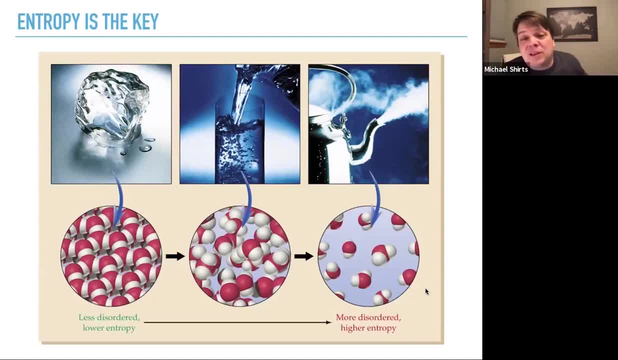 Whereas liquid water, you've got hydrogen bonds being formed a lot of the time, but the molecules slide past each other. And finally, in steam, the molecule are behaving like a gas and they're not interacting with each other very much. they're. 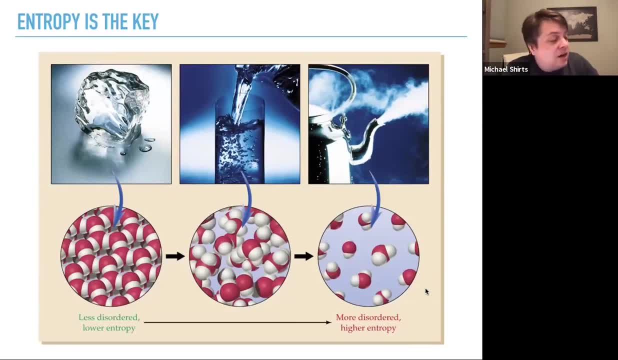 completely free to move around. So that is more distorted and higher entropy, And so the phases usually see a series: solid is the low entropy phase, liquid is a medium entropy phase and gases are a high entropy phase. So let's revisit that reaction about what's going on. So if we actually 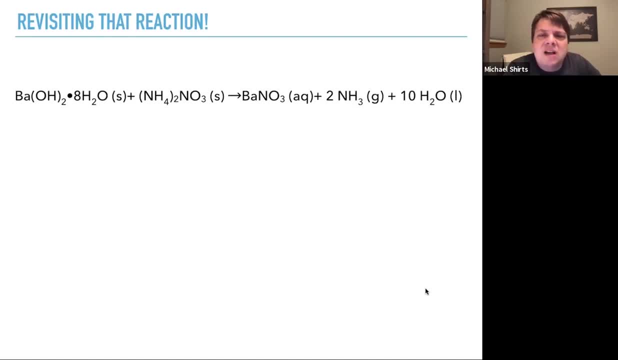 put the phases in. remember, this is a reaction where you mix together two solids and it became like a slurry, because what would happen is you'd got, you have barium nitrate, but you also had ammonia gas being released and H2O liquid being released as well. So it was going from something. 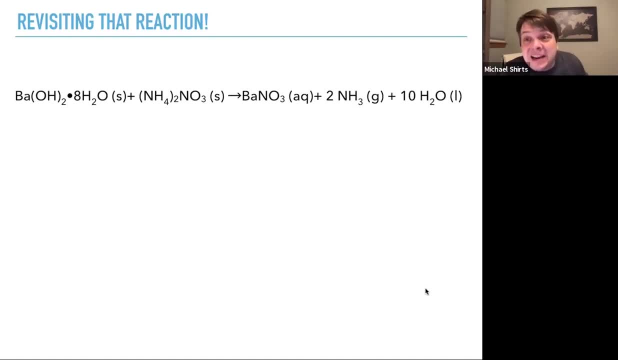 that was entirely solid to something that had a lot of liquid and gas as well, And like a solvent, an ionic solvent dissolved in liquid. that's pretty disordered as well compared to solid crystals. So the two factors are energy and entropy. Processes proceed to lower energy. 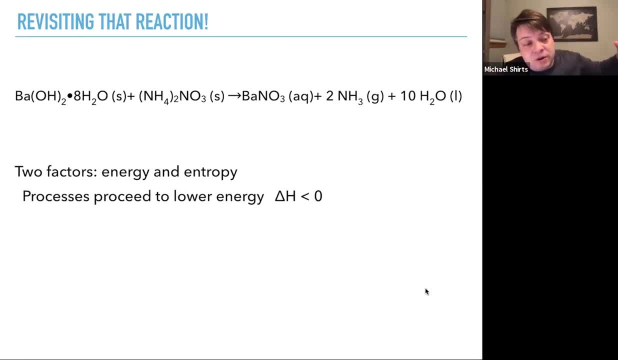 delta H is less than zero. If a system is exothermic, it will tend to go proceed in that direction. Some exceptions we'll talk about later. And processes also proceed to more disorder when the entropy increases. So either when the enthalpy decreases or the entropy decreases- We won't talk about exactly how to. 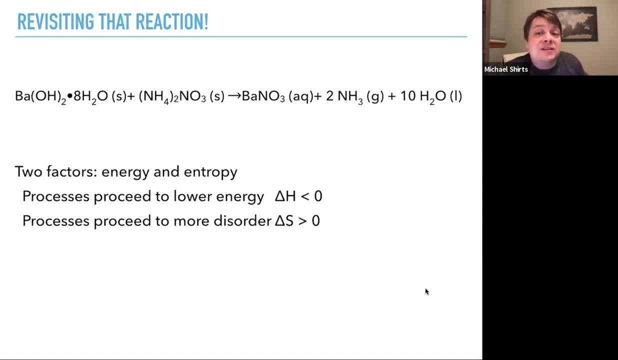 combine them. What if the entropy increases but the enthalpy also increases? What do we do in that case? We'll talk about that next time, about how to balance. But those are two effects that can push a reaction forward. The fact that it's it lowers in. 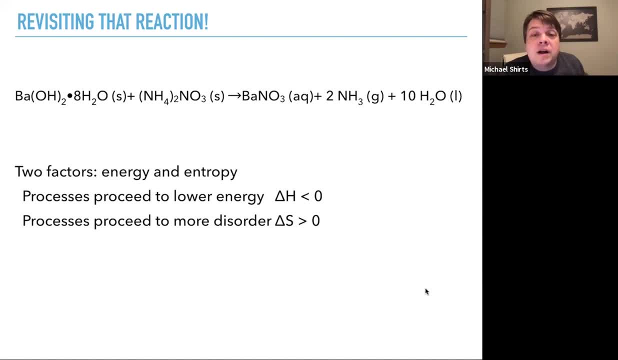 becomes lower in enthalpy, ie it's exothermic, or that it increases in entropy, So yeah, So in this case we start with. all solids end up with gases, liquids, ions dissolved in water, definitely a higher entropy state, And that high entropy is enough to compensate for the fact that it is. 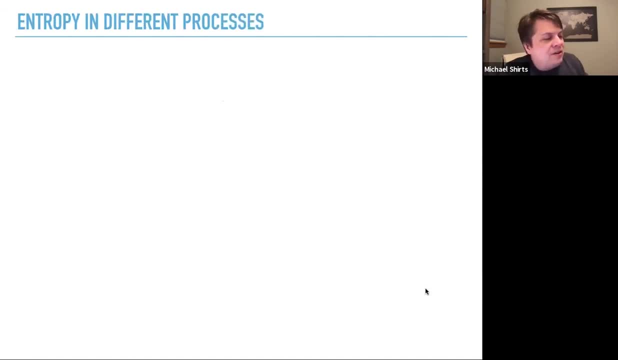 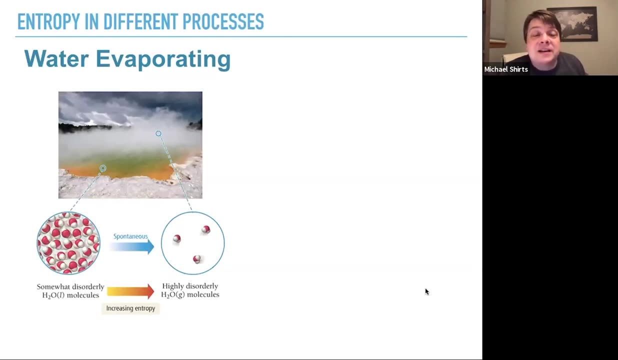 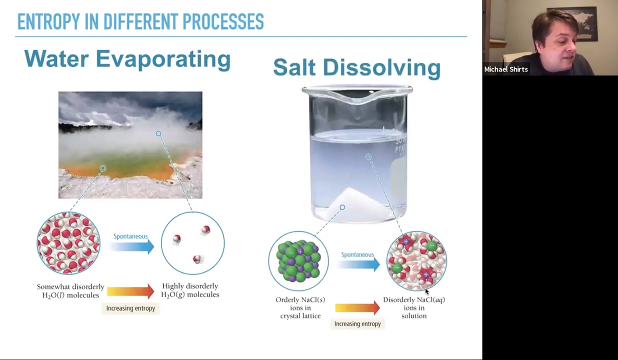 an endothermic reaction. Okay, So entropy in different processes. So if water evaporating is a good case, you need to take a thermal energy in, And when that happens, if it, if it's hot enough, it'll spontaneously vaporize. or salts ions dissolving in salt. You go from order orderly. 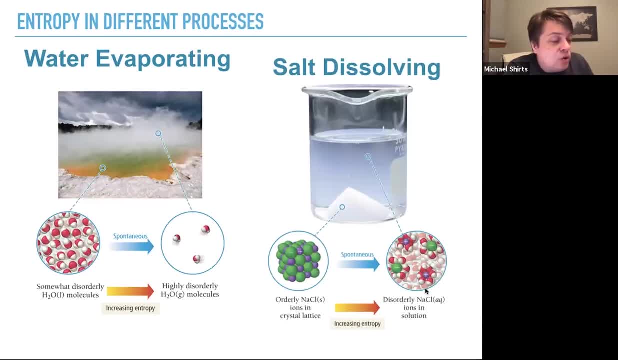 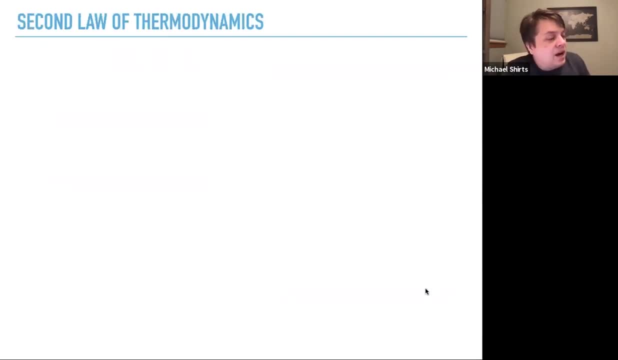 sodium chloride ions at a crystal lattice to disorderly being dispersed throughout the entire solution. So clearly there is a loss of order there. So so now we want to sort of revisit and go back to the second law of thermodynamics, law. one phrasing of it: you can't win. uh, you cannot. the energy is conserved. but the second law is: 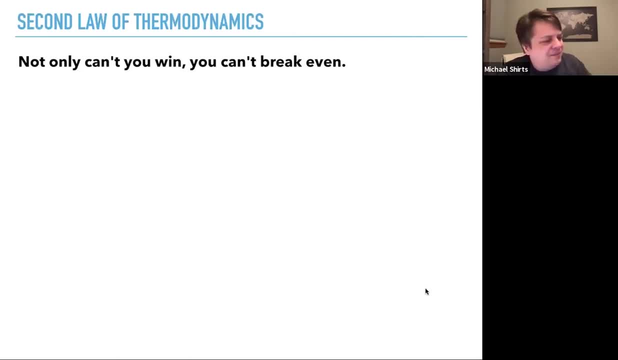 that, uh, not only can't you win, you can't even break even. um, that reactions receive, proceed to spontaneously in the direction that increases the entropy of the system plus the surroundings, and, uh, so the entropy of the universe increases and spontaneous process. so spontaneous process again proceeds on its own without any continuous external influence. a non-spontaneous process takes. 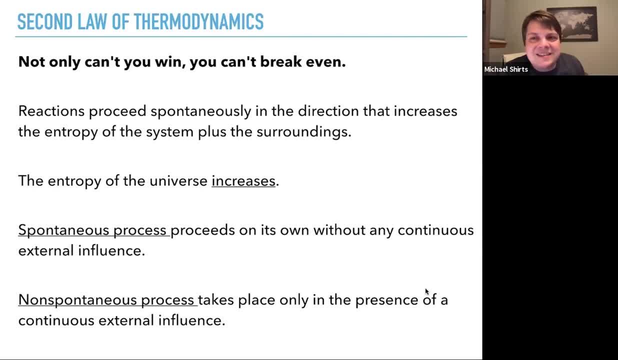 place only in the presence of a continuous external influence. so that's the uh, the key is the uh, the entropy increasing. so entropy increasing uh, all processes uh incur a total increase in entropy. um, if the system plus the surroundings, sometimes the system might decrease in entropy, but it will be accompanied by a increase in the entropy of the surroundings. so, um, some, 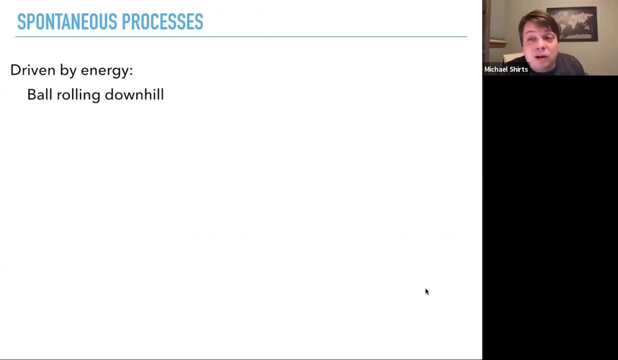 spontaneous processes that are driven by the energy. a ball rolling downhill. it's losing potential energy, uh metals oxidizing, iron rusting or copper grain gaining your green patina because the uh, the uh, copper and iron oxygen bonds are stronger than the bonds inside the metal. uh gas is dissolving into liquid. right, they don't have. 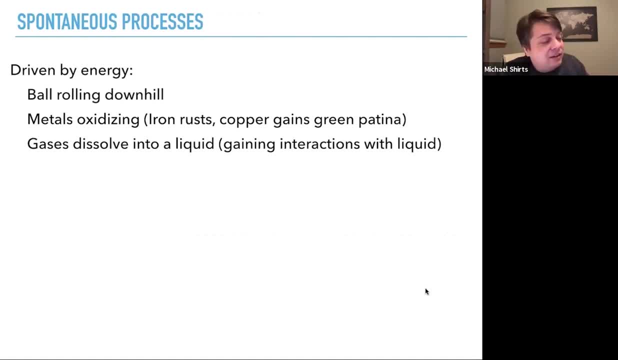 interactions outside, but then, when they interact with the liquid, they gain interactions um. water freezing into ice at low temperature- uh, that happens is spontaneously because of the um, the ability to form the hydrogen bonds. uh, but driven by entropy, a gas dispersing from a small container to a low container, diapersonal. 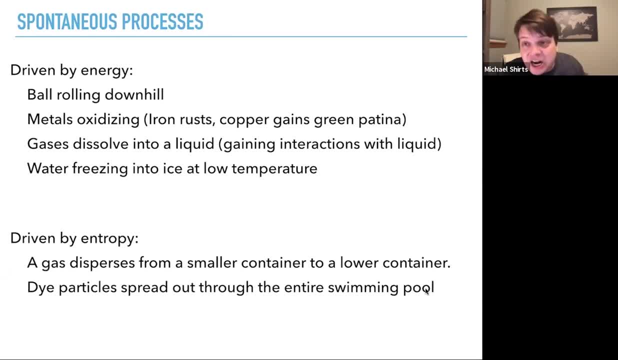 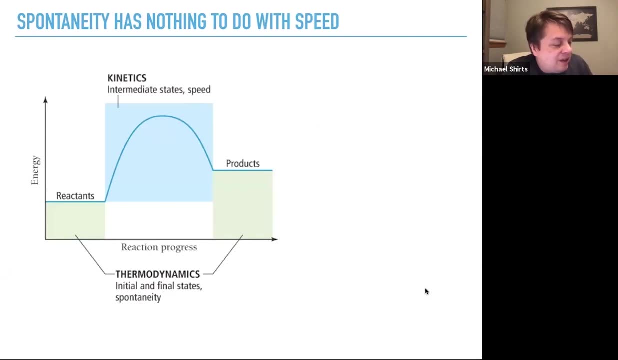 particles spreading out if they're dropped in, spreading out through and through like an entire swimming pool until it's completely dispersed. a hot system reaching thermal equilibrium with the environment. that is also a process that is driven by entropy. uh, one important thing here is that spontaneity has nothing to do with speed. so we think of the reactants, the products, of course. 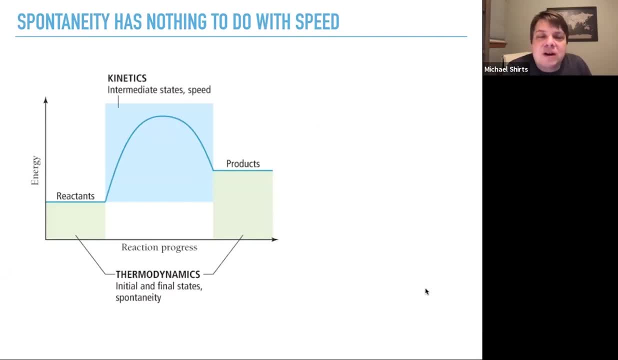 the kinetics are determined by the intermediate states, and those describe the speed at which the reaction occur, but whether it's spontaneous or not is solely a measure of its initial and its final state is that this reaction is a process of the reaction that is driven by the environment, and so